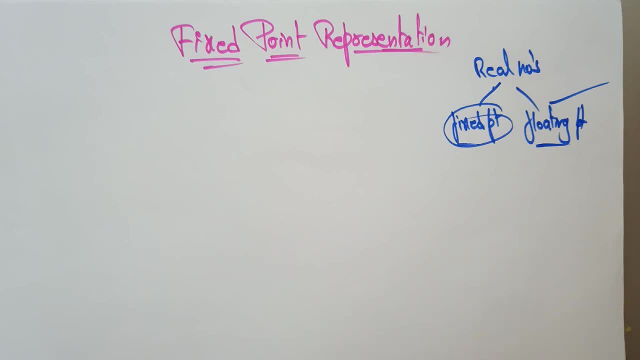 Only, even though we are working on the floating point representation, you have to know the concept of what is fixed point and what is floating point also. Okay, so let's have a clear idea on fixed point. Later we can see the floating point. Now let's start. So, fixed point, What is a fixed point representation? A fixed point representation means there is a fixed number of digits after a decimal part. So, whatever the decimal part you are, taken that that means. 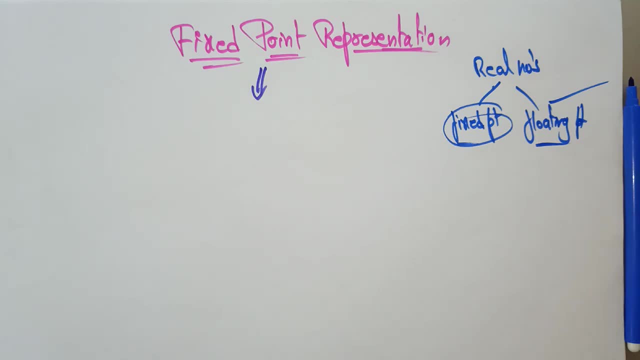 a binary point will be there. that should be fixed. You can't move that point. Okay, you can't move that point. that the let me write this: There is fixed number of digits, a fixed number of digits after decimal part. After decimal part, there should be a fixed, fixed number of digits will be there. You can't change that, the fixed number of digits, Whereas in the floating point you can move that point. 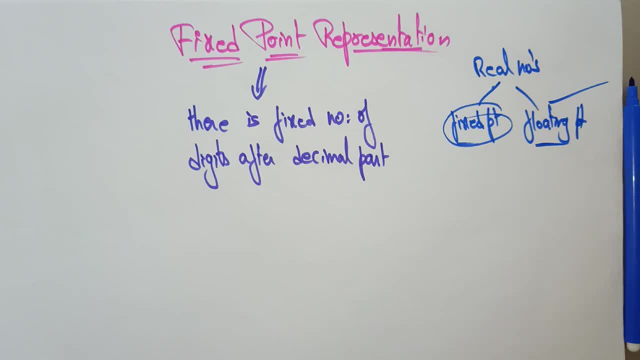 move the base point, that is a decimal part, to the wherever you require. okay, that is the decimal binary point, you can be move that, but here in the fixed point representation you can't change, it is fixed. okay, the binary point is fixed. now let's work on this: the fixed point representation. 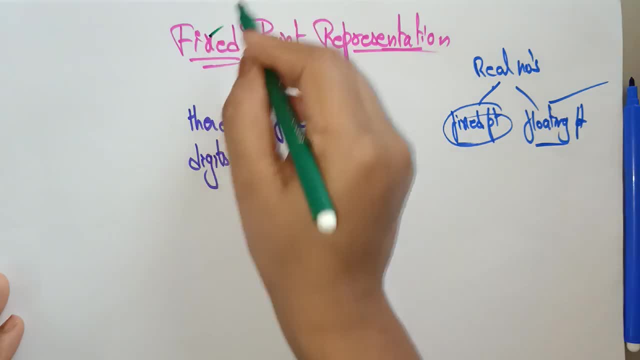 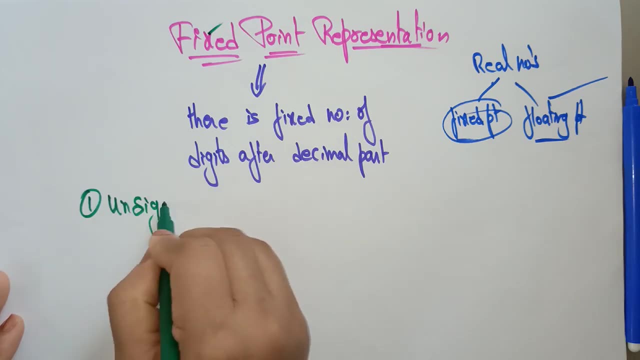 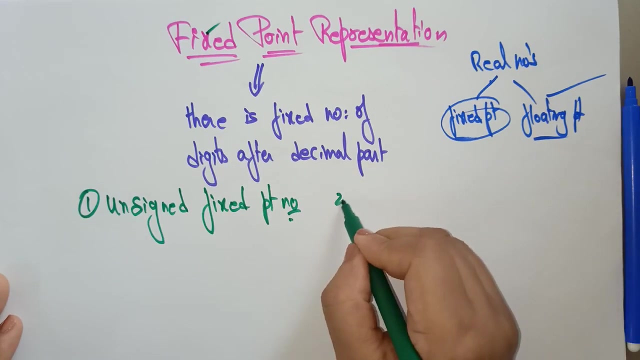 is of two types. we are discussing fixed point representation. it is you can represent the fixed point in two different way. one is a unsigned fixed point number, unsigned fixed point number, and the next one is a signed fixed point number. so if it is unsigned means no problem, positive number. positive number means you can work on. 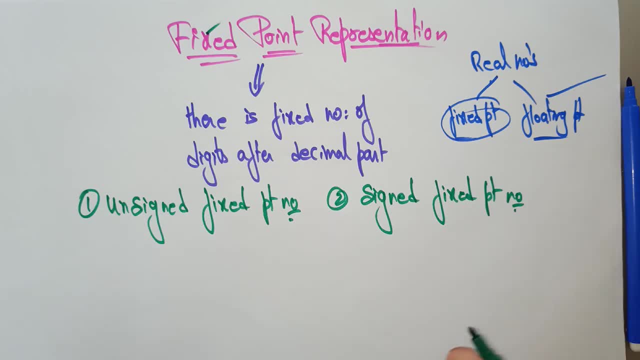 directly. okay, no, nothing will happen. it's just like in normal numbers. so the problem is rise whenever we are working on the signed fixed point number. so the unsigned fixed point numbers is again. divide can be represented in two ways. either you can represent it in twos complement or other you can, or else you can follow the another method. 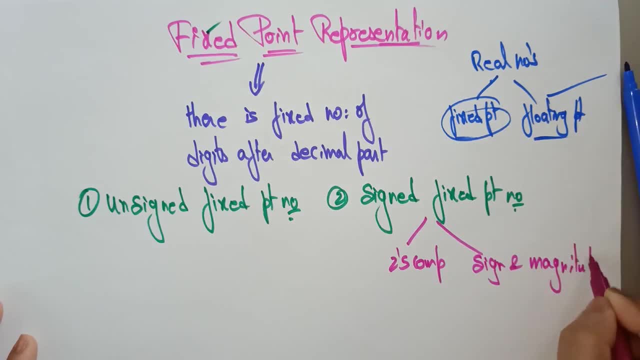 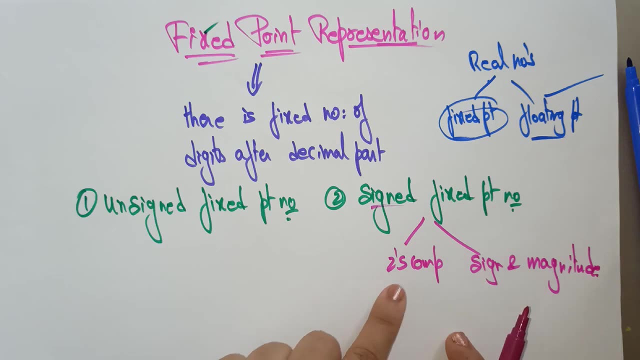 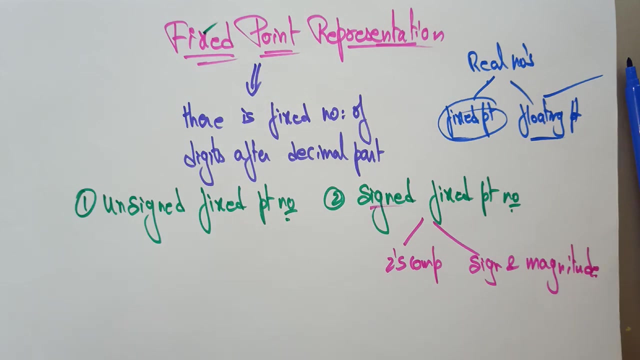 sign and magnitude method. okay, if the sign numbers are there, that means, if the negative numbers are there, you have to represent the fixed point in twos complement or else in the sign and magnitude representation. if unsigned fixed point, then there is no problem with that. so here i'll. 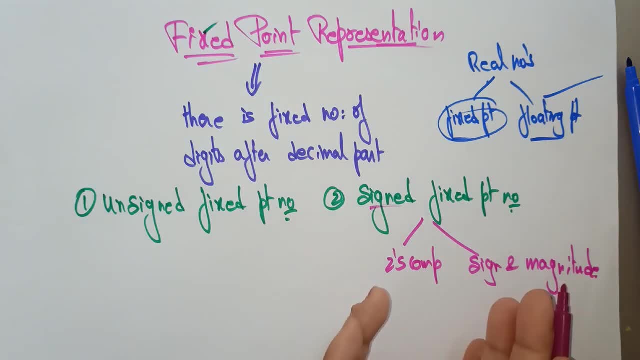 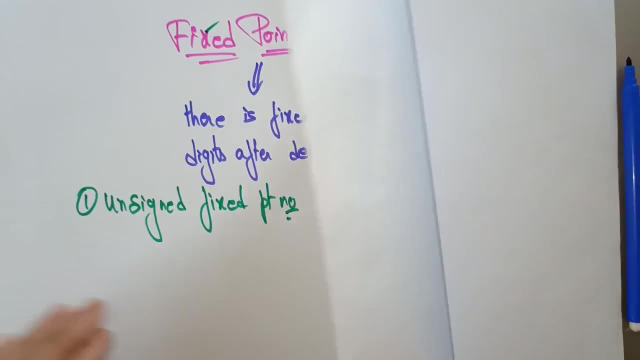 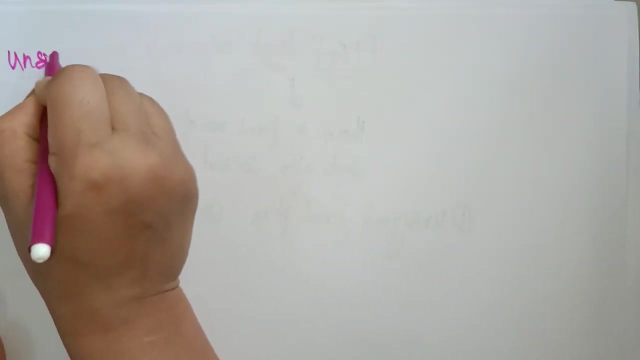 just explain you what is an unsigned fixed point and the signed fixed point, with an example. in the next video i'll take more examples to work on that fixed point representation. okay, now let's start with the unsigned fixed point representation. so i already said, unsigned means it's a positive number. unsigned. 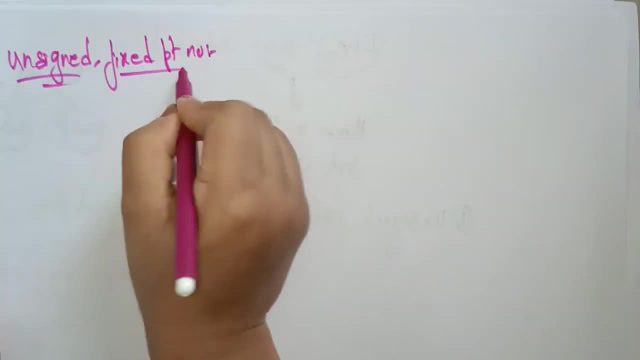 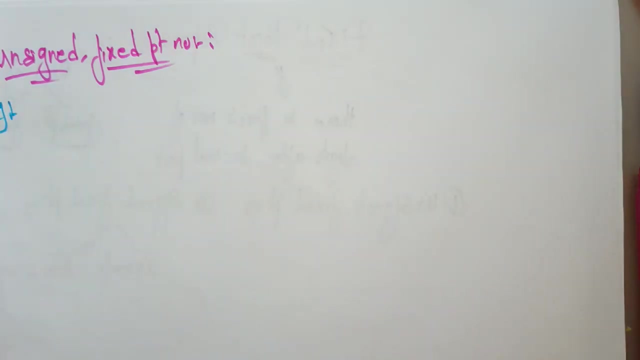 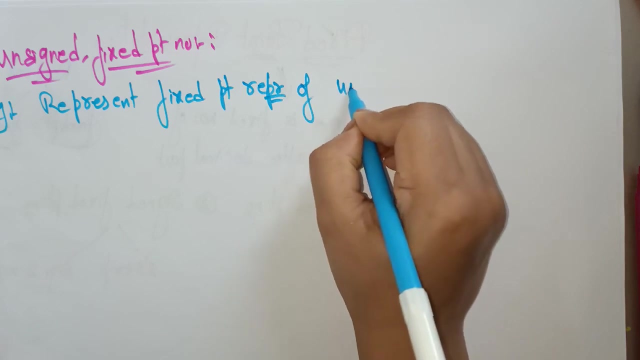 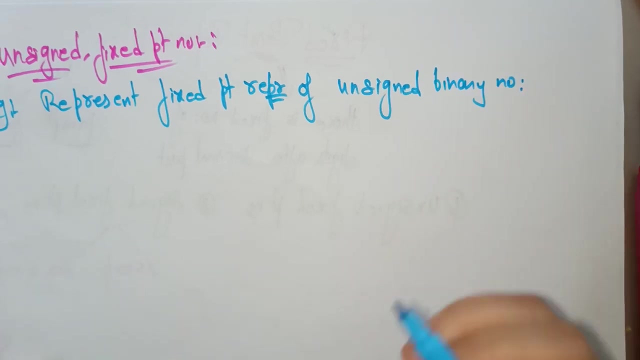 fixed point number. oh, here i'll take simple example to explain this: unsigned fixed point number to represent a fixed point representation of unsigned binary number. let me write the question represent: they are asking to represent a fixed point representation of unsigned binary number. so they are giving some binary number which is an unsigned. they are mentioning it is an unsigned. 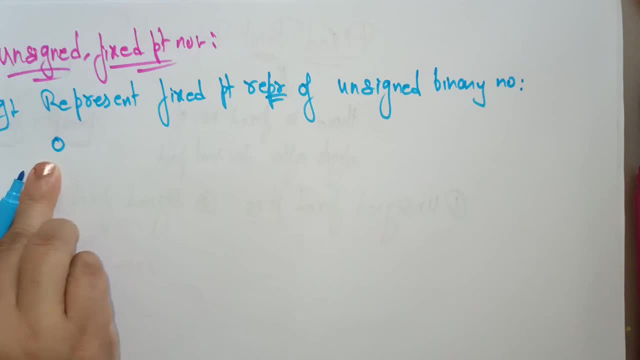 unsigned means the most significant bit should be zero one one, zero one, one, zero. so they are said that it is an unsigned binary number they are asked to represent in a fixed point representation. the given number should be represented in a fixed point representation. so they'll give some condition like using four integer bits and three fractional bits. 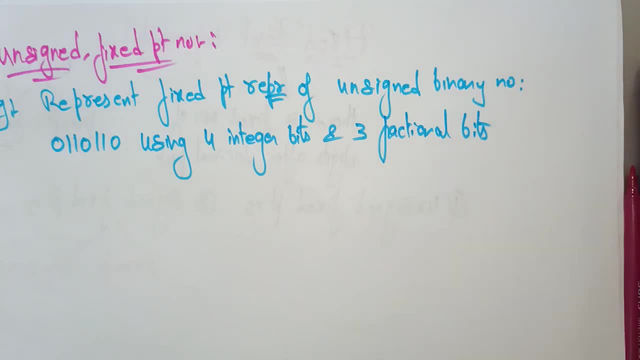 so. So this is a question they are given. They are asking us to represent a given binary number in the fixed point form. Before going to explain this problem, I want to explain you. whatever the number that is there, that number can be divided into three parts. One is the sine part and next is 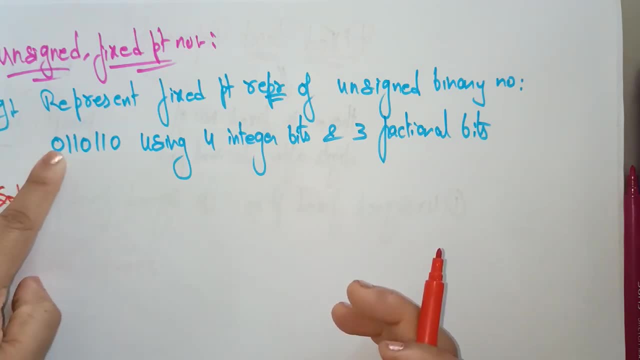 integer part and next is a fractional part. Sine part means the most significant bit. whatever the starting bit is there, that goes to the sine part, and next parts can be divided into integer part as well as a fraction part, So they are given as a condition. You have to represent this unsigned. 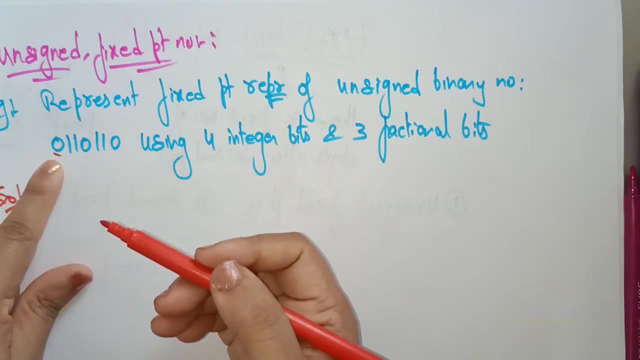 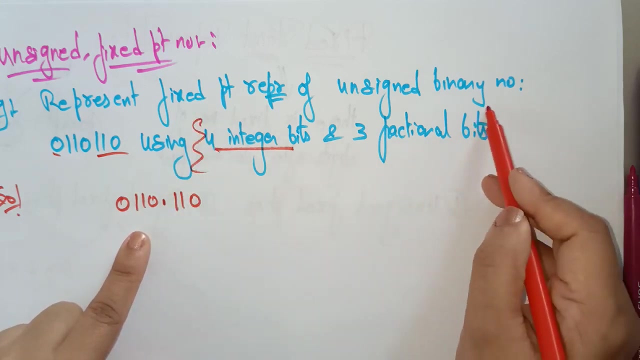 binary. Unsigned binary means the starting most significant is zero only. Okay, there's zero and four integer parts. Integer part is always included with sine bit is always included with sine bit. So 0, 1, 1, 0 dot. this is the integer part and three factional parts: 1, 1, 0.. So this condition is saying: